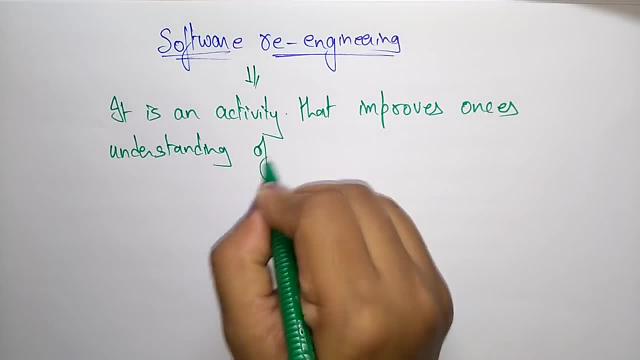 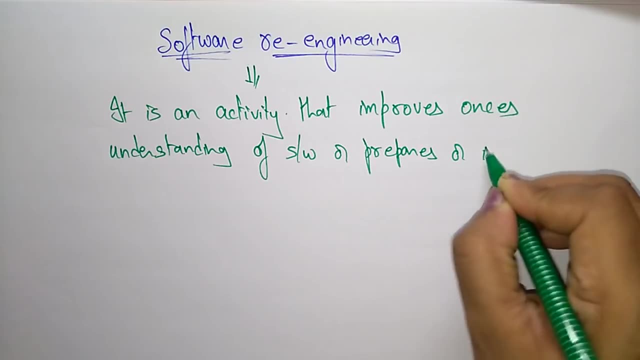 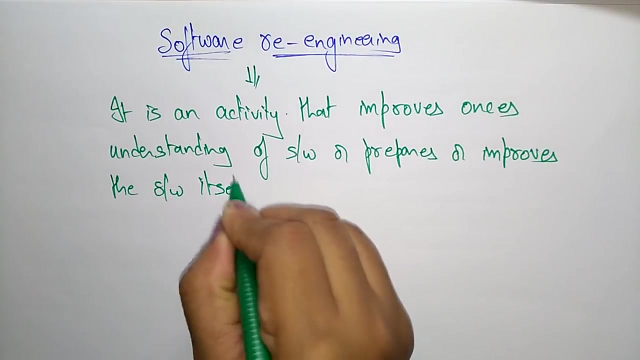 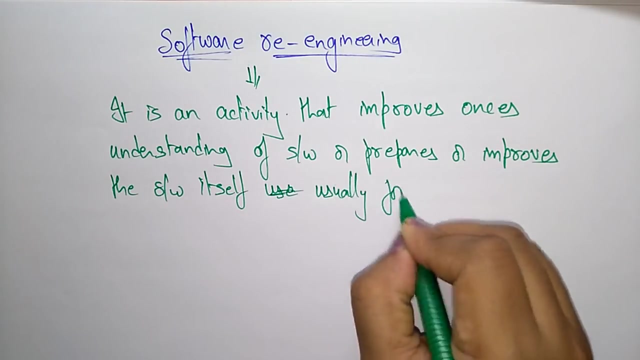 One's understanding of software, or prepares or still improves, improves the software itself. Useful for usually, usually for increased maintainability, Maintainability, reusability, evolvability. So what it is saying that? Now let us see A software re-engineering. it is an activity that improves one's understanding of software. 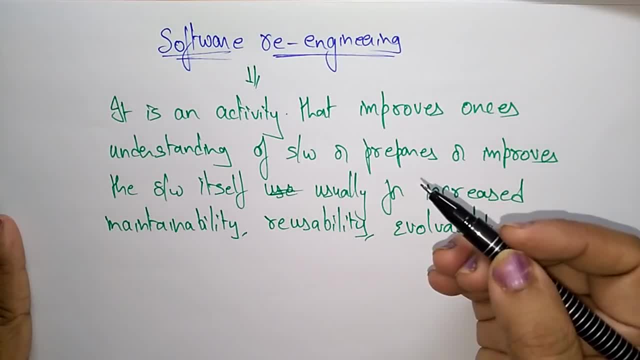 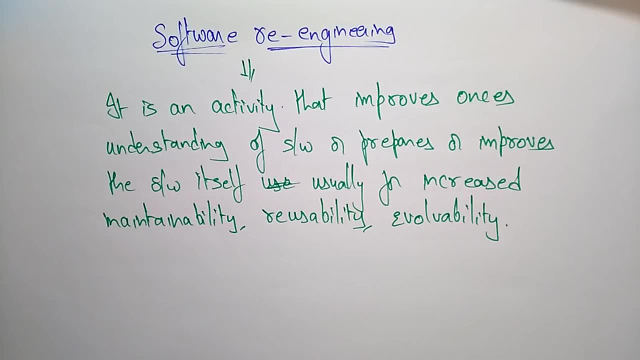 Mainly, the use of re-engineering is to understand the software or to prepare the software or to improve the software. Usually, for why we are improving the software and why there is a requirement to understand the software, Because of increasing the maintainability, reusability and evolvability- we are using the software re-engineering process. 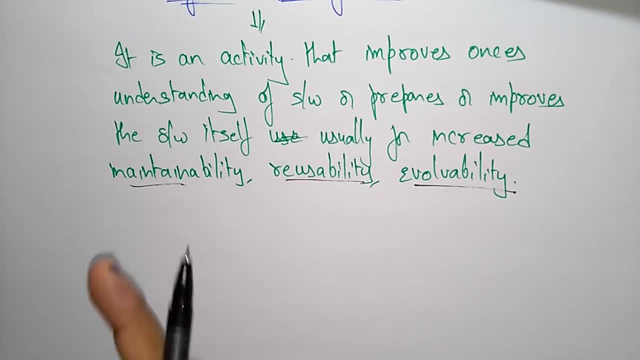 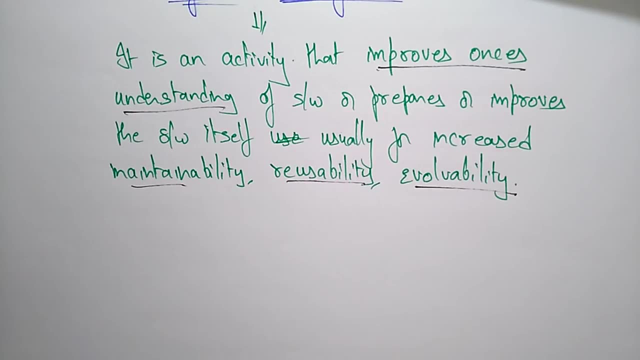 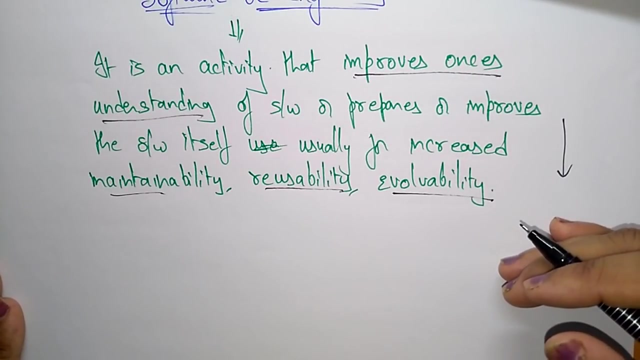 Okay, I understand that software re-engineering is nothing, but it is helpful for improves the one's understanding of software. So how we are doing this? software re-engineering? Forward engineering means Going forward by taking specifications and try to implement the project. 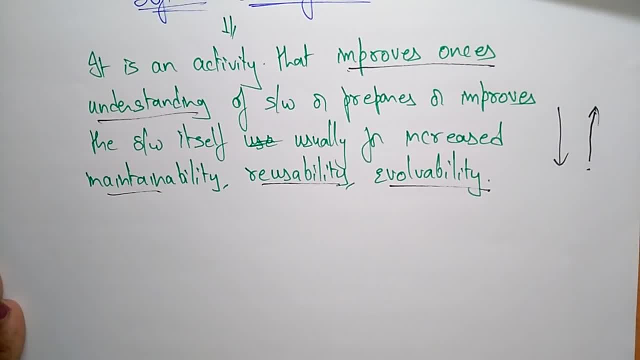 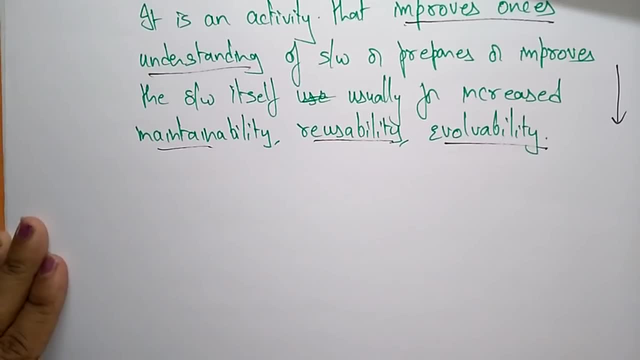 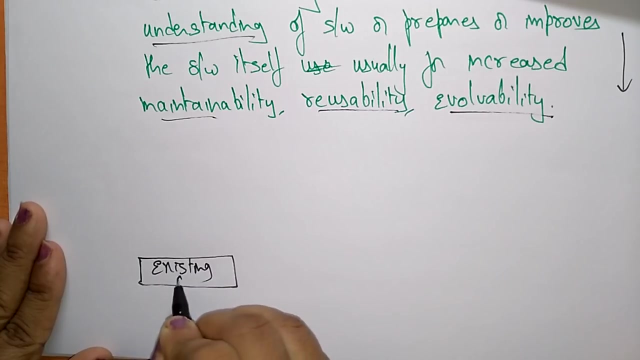 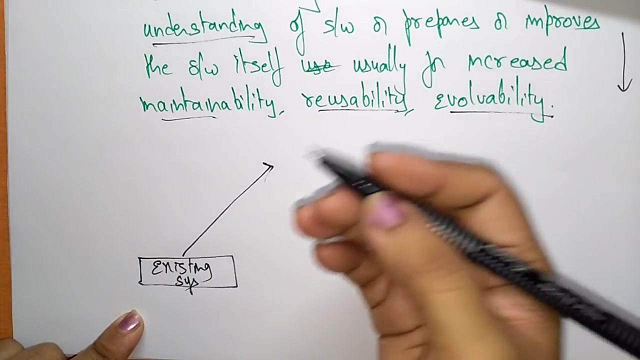 Reverse engineering means with the help of the code we are trying to find out the problems. means we will reach to the documentation stage. Then what is software re-engineering? The software re-engineering is done is nothing, but you have to take the existing system. means already developed a system. you have to take the existing system. try to go back. 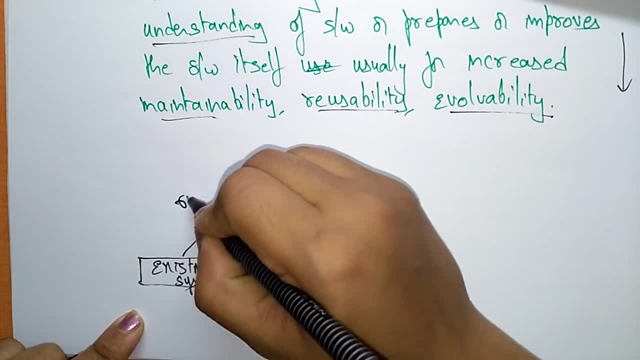 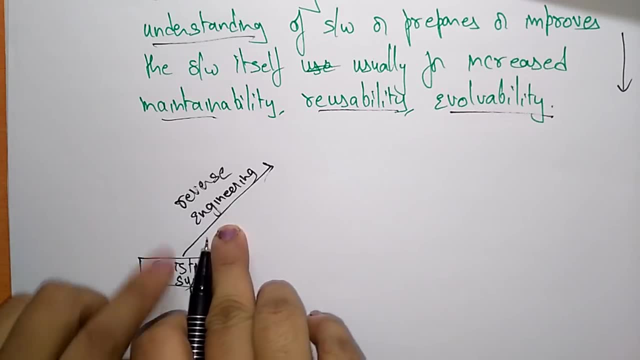 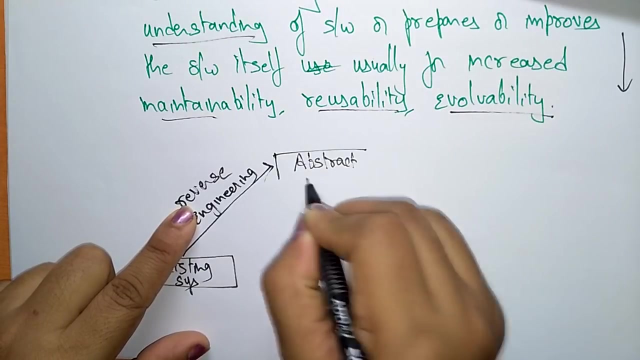 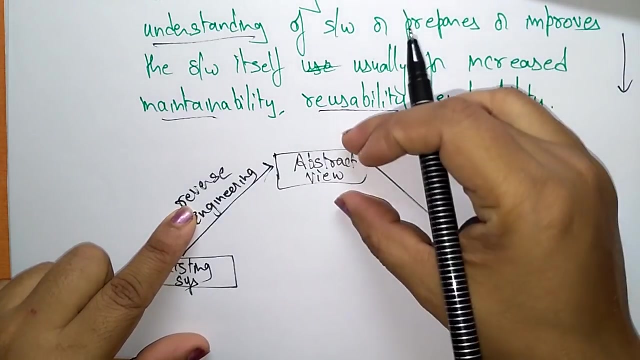 Go back means it is nothing but reverse engineering. You follow the reverse engineering strategy here in one phase. take the existing system, follow the reverse engineering strategy. You will get an abstract view, abstract view, and you will- you have taken the abstract view and start to use the forward engineering technique here.